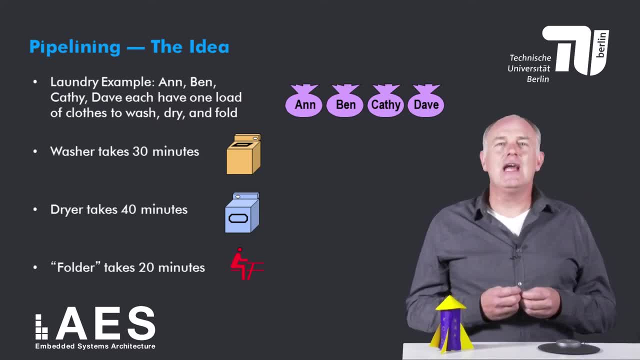 the issue, the problem of doing several laundries. In particular, the computer engineering students Ann, Ben, Kathy and Dave each have a load of clothes to wash, dry and fold. Furthermore, the washing machine takes half an hour. 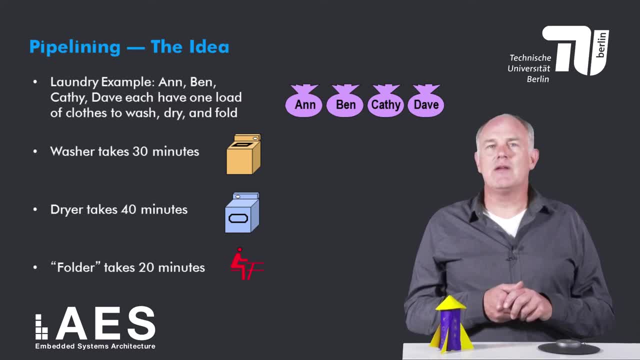 the dryer takes 40 minutes and the folder takes about 20 minutes. Unfortunately, there is no folding machine yet, and in my home it's usually me taking care of this task. Let's see how much time it takes to do these four laundries. 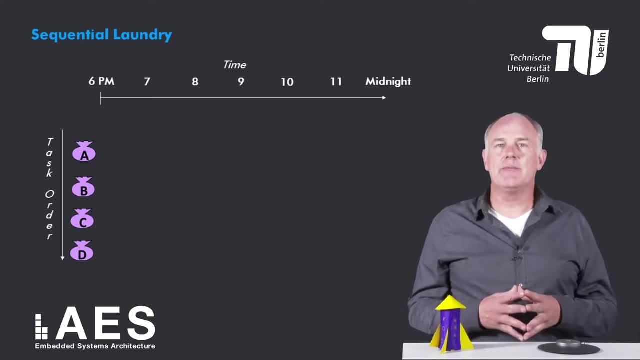 one after the other when we start at 6 pm in the evening. Here time is shown horizontally from left to right, and the four tasks, the four laundries, are shown vertically from top to bottom. We start by the first laundry at 6 pm. 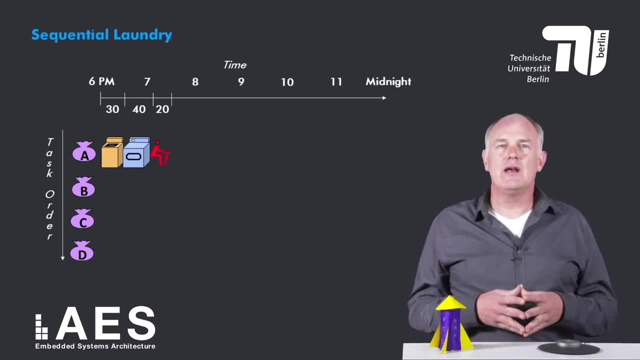 We wash it, we dry it and we fold it. this in total takes one and a half hours and we're done with the first laundry at 7.30.. Then we start our second laundry. we wash it, we dry it, we fold it. 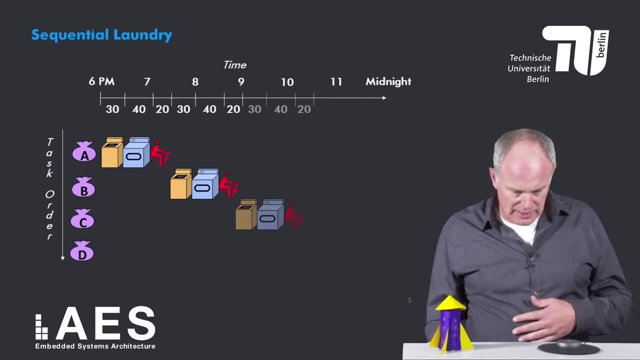 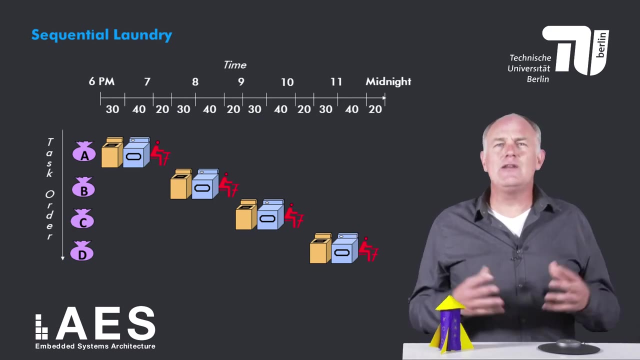 and we're done at 9 pm with that. Then we start our third laundry. third laundry: again we wash, dry and fold and we're done at 10: 30.. at that time we start our fourth and final laundry and we will be done at midnight. then unfortunately it's too late to go to a party. 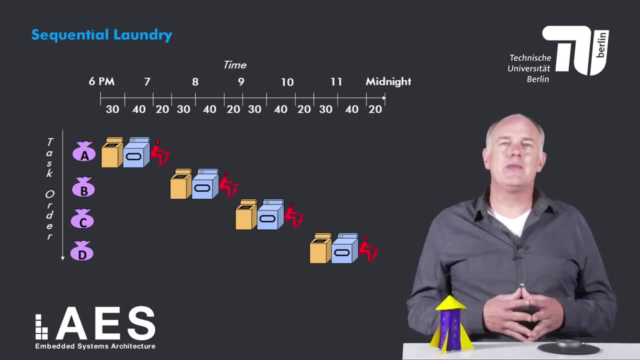 since our class on computer architecture starts tomorrow at 9: 00 am. but wait a minute, aren't we doing something- let me put it this way, not so smart? since the washing machine is done at 6: 30, wouldn't it make more sense to start the second laundry at that time, instead of waiting until the 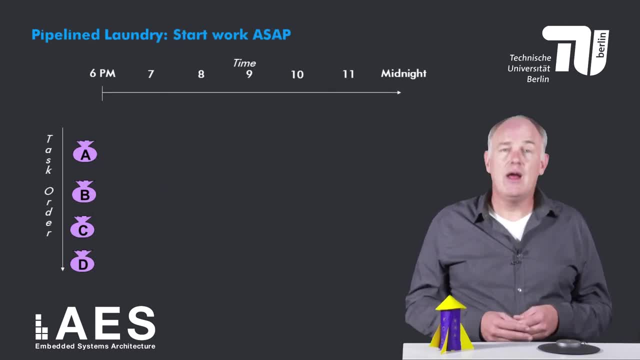 first laundry has been folded. that's the basic idea behind pipelining. start working on the next task, in this case laundries, as soon as possible, as soon as a resource- in this case washer, dryer or folder- capable of performing that task becomes available. let's see how this will look like. 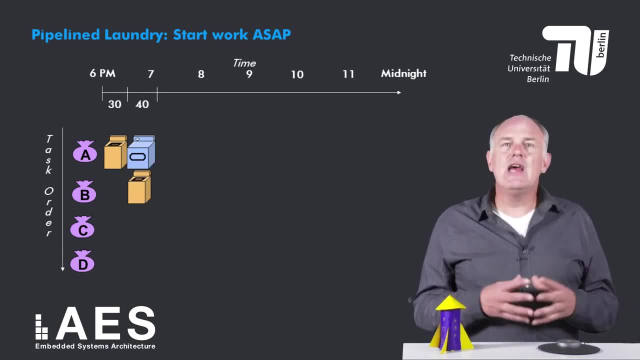 first we wash laundry a, then we dry laundry a and at the same time- because the washing machine has become available- we wash laundry b. then, at the same time, we fold laundry a, we dry laundry b and we wash laundry c. now laundry a is completely done. similarly, after we fold laundry b, we dry. 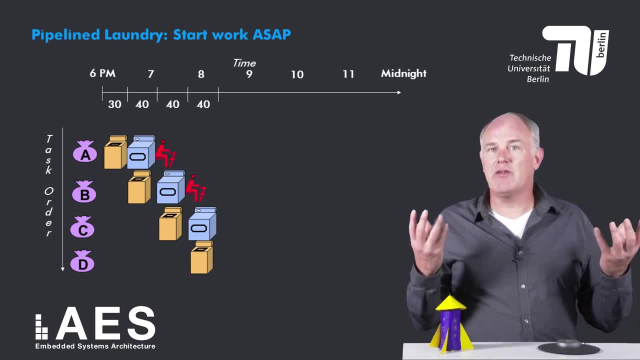 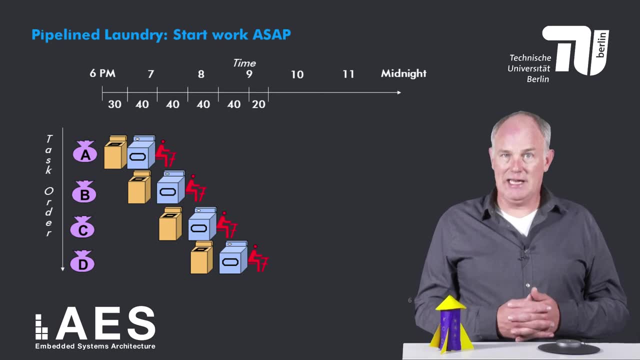 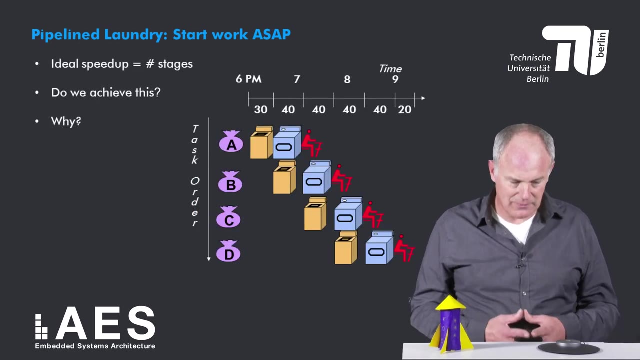 laundry c and we wash laundry d in parallel simultaneously, and so forth and so on. now we are done at 9: 20.. we still have time to go to the party and to be on time for class tomorrow. in the ideal case, the speed up we obtain thanks to pipelining is equal. 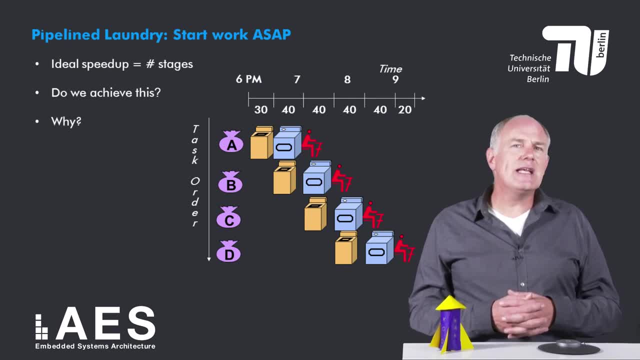 to the number of stages. do we achieve this? in this case, the answer is unfortunately no. our sequential laundry took from 6 pm to midnight, so six hours, or equivalently 360 minutes. pipelined laundry, on the other hand, takes from 6 pm to 9: 20, so 3 hours and 20 minutes, or equivalently 200 minutes. 360 divided by 200 equals 1.8, so no. 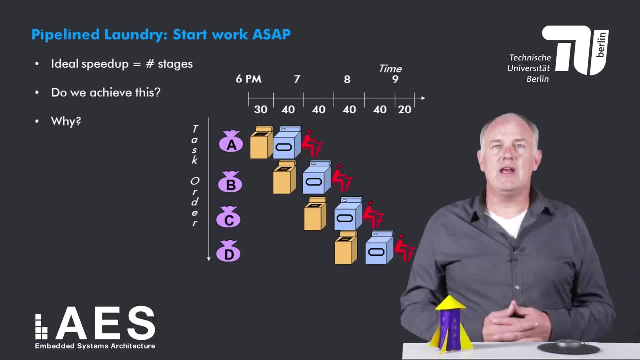 we do not achieve a speed up of 3, corresponding to the number of stages. there are two reasons for this. first, there's a startup effect. it takes some time for the pipeline to fill up. if there would be an infinite number of laundries, a laundry would complete every 40 minutes. compared, 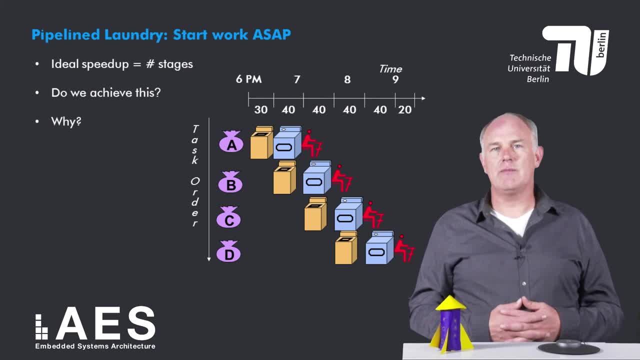 to 90 minutes in the sequential laundry case. so then the speed up would be: 90 divided by 40 equals 2.25. this is somewhat better, but still not three. so the second reason why the speed up is less than the ideal speed up is that the stages take different amounts of time. drying takes 40 minutes. 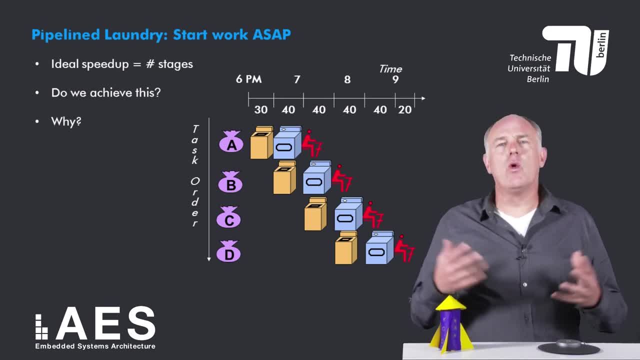 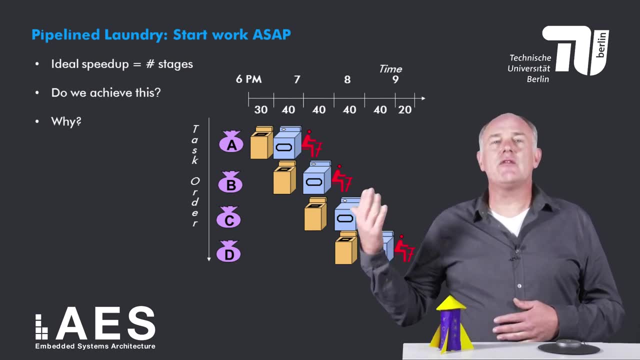 washing takes 30 minutes and drying takes 20 minutes and folding only takes 20 minutes. because there is only one dryer, it cannot start drying the next laundry until it has finished drying the current laundry. also, the folder cannot start folding a laundry until the dryer has dried that laundry. for this reason, a bit of time is lost in every stage.